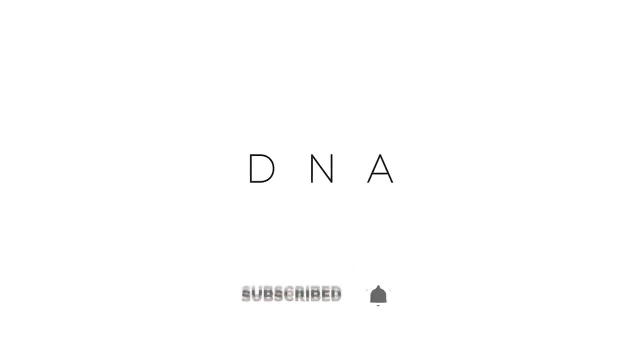 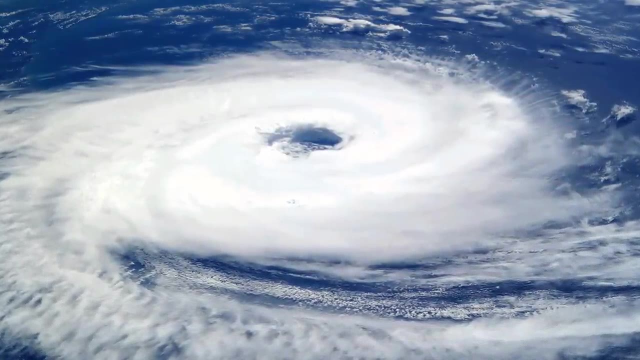 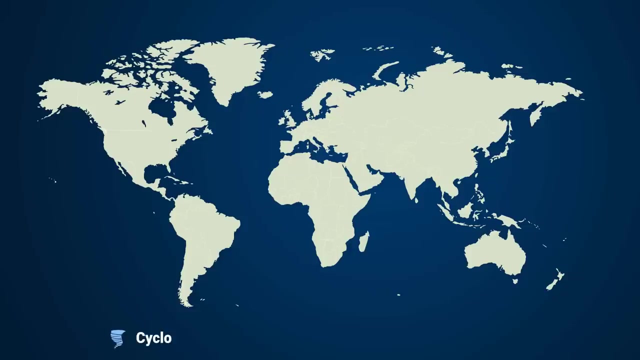 subscribe to DNA so that you don't miss out any of the new videos that we post. Cyclone is a general term used by meteorologists to describe any rotating organized cloud that originates over waters, For example cyclones, hurricanes or typhoons. One event, but different names. 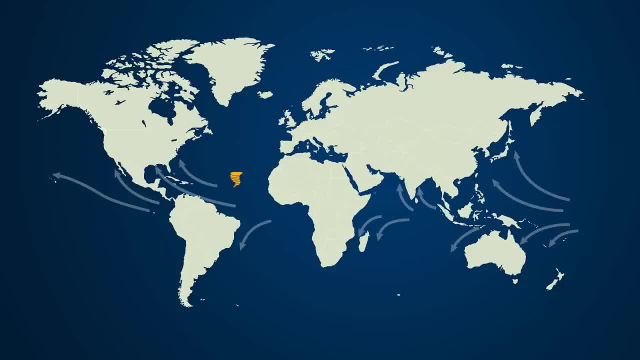 depending on the location. In the Atlantic and the northeast Pacific it is called a hurricane, And in the northwest Pacific it is termed a typhoon, and in the South Pacific and Indian Ocean it is called a cyclone. You can also classify them based on Similarly hemispheres. 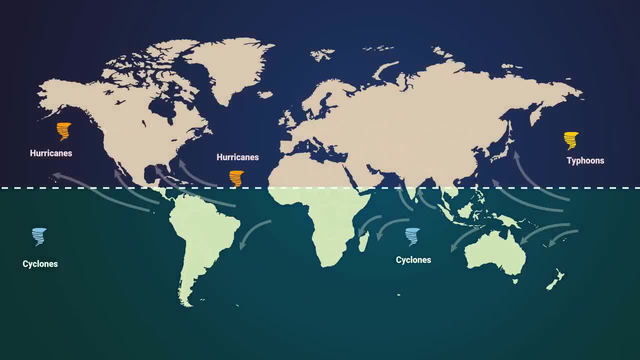 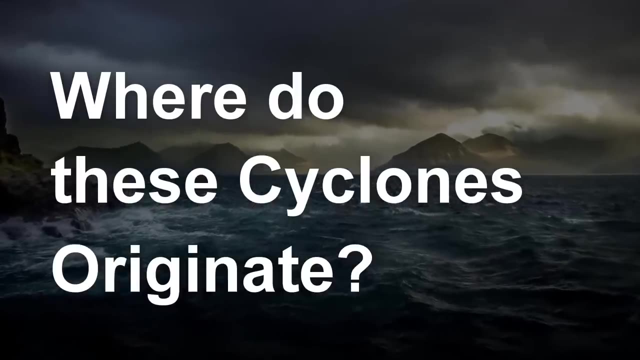 The northern ones as hurricanes and the southern ones as hurricanes or typhoons. ones are cyclones. there are also a few other differences in them, apart from where they originate, like the cyclones are usually clockwise, but the hurricanes are usually counterclockwise. where do these cyclones originate? when the atmospheric pressure is low over a large water. 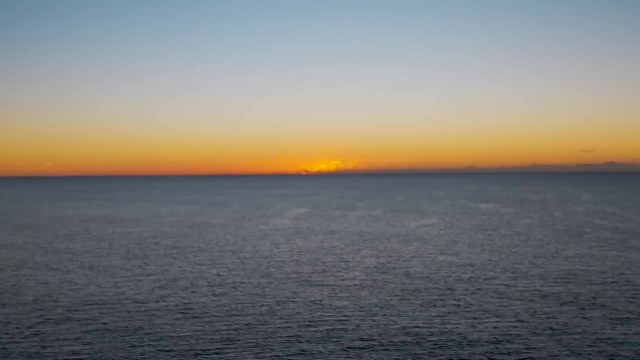 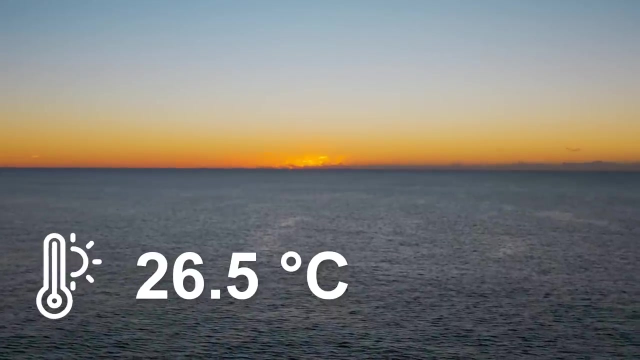 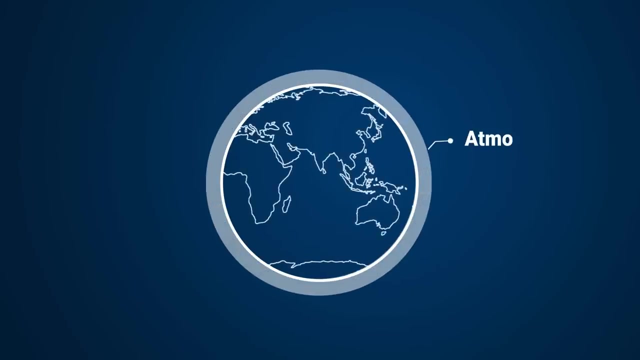 body that is still and the temperature of the water is more than 26.5 degrees celsius, then they form into a cyclone. before getting into any deeper, let us understand what is atmospheric pressure. in general terms, the density of air in our atmosphere differs from place to place. 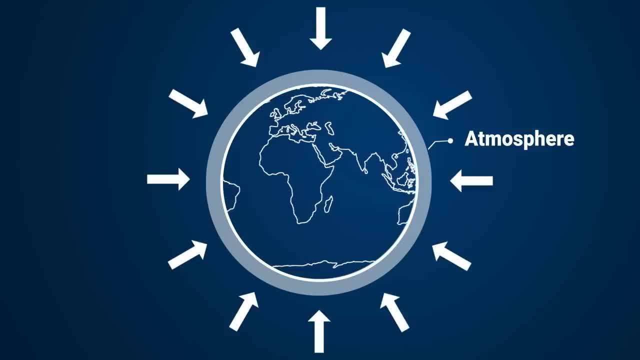 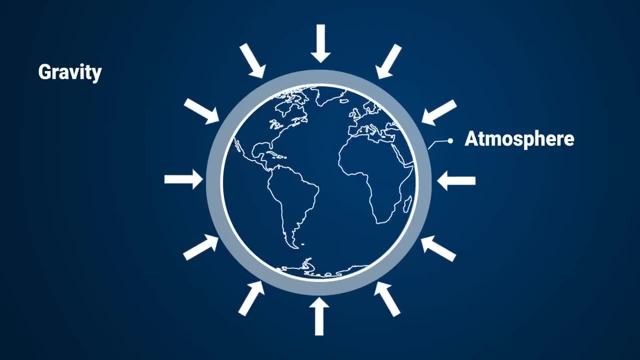 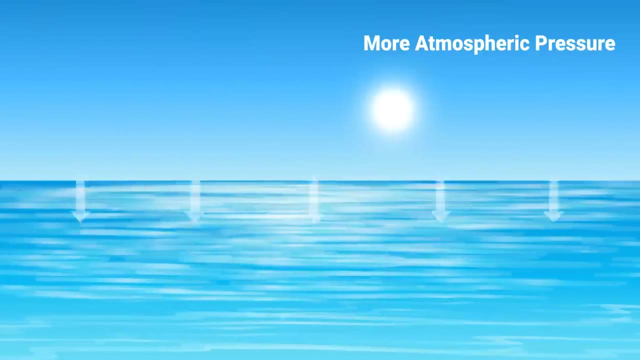 they are not the same everywhere. atmospheric pressure is the weight of air acting against the surface of the earth. along with gravity, air in the atmosphere creates a pressure on earth's surface called the atmospheric pressure. atmospheric pressure is more on the earth's surface and as we move upwards there is less amount of air and hence the 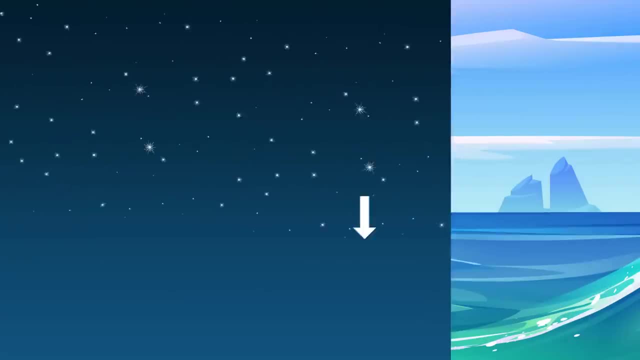 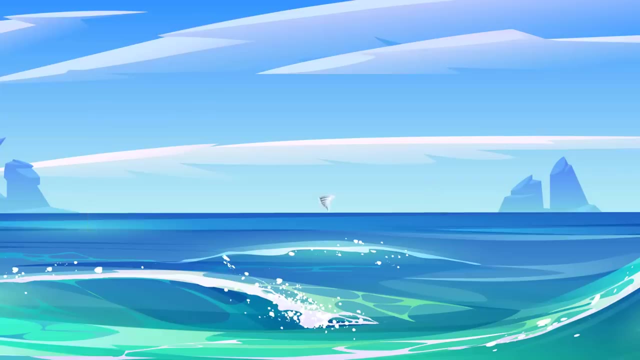 atmospheric pressure decreases. when there is low atmospheric pressure on a large water body on earth's surface, they turn into a cyclone. this process of thin air circulating, strengthening and developing into a cyclonic formation is called cyclogenesis. so how does it become a huge stormy? cloudy cyclone. when the atmospheric pressure is low, the warm air rises to fill the gaps and the cold air goes down as they have moisture in it. the warm air: as it reaches the place, it becomes more warm and it rises rapidly, thus creating more gap. so the surrounding air rushes in to fill the place.